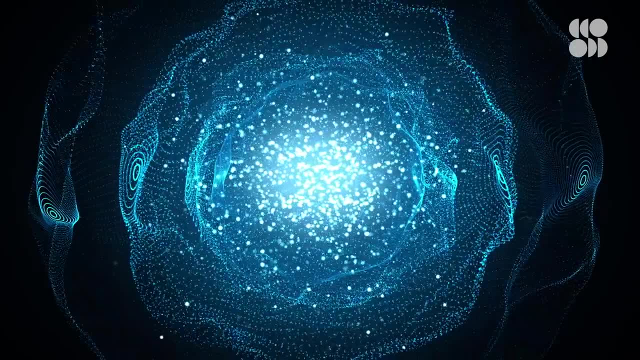 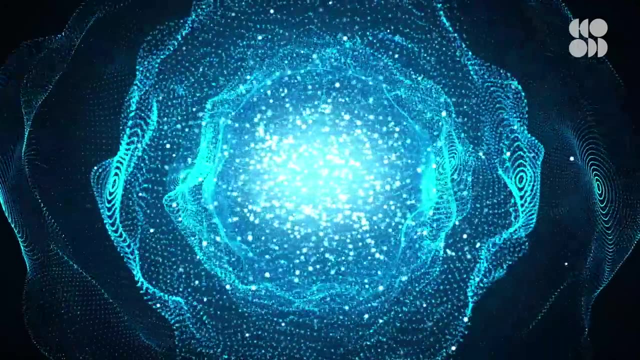 This is an experiment that allows us to see from the wobble of the muons what's otherwise: an invisible quantum world that contains all kinds of stuff that we'd like to know about, So it's basically potentially pointing us to something that we don't understand. 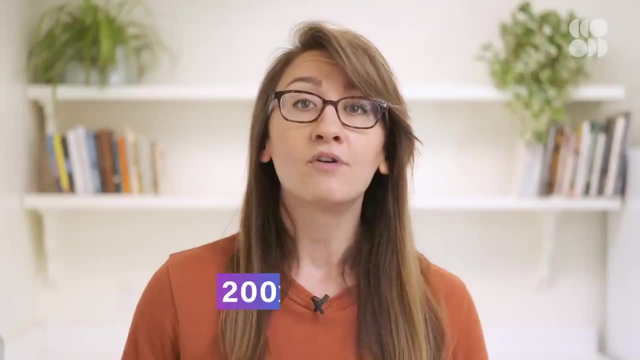 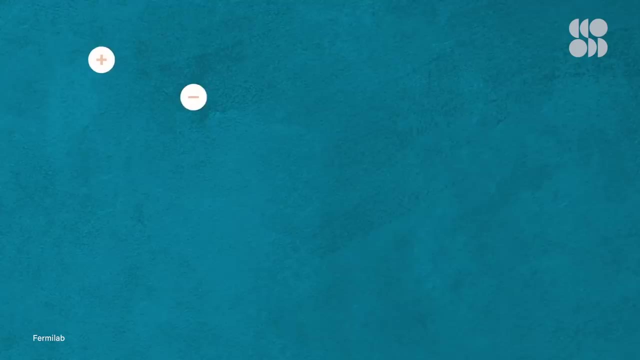 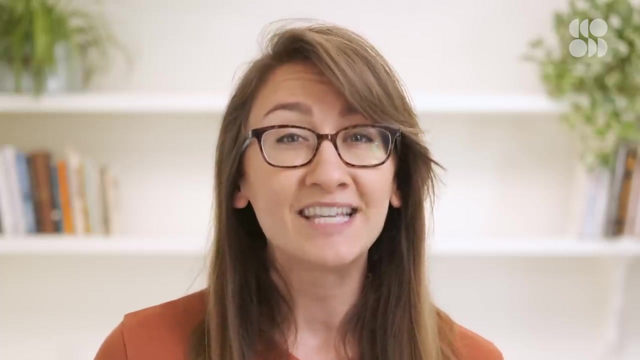 and this is why it's very interesting. Muons are around 200 times heavier than electrons, which means the moment they become magnetic is 200 times smaller and therefore way more sensitive to all of the virtual particles swimming around in the quantum realm. So to measure this moment, precision is. 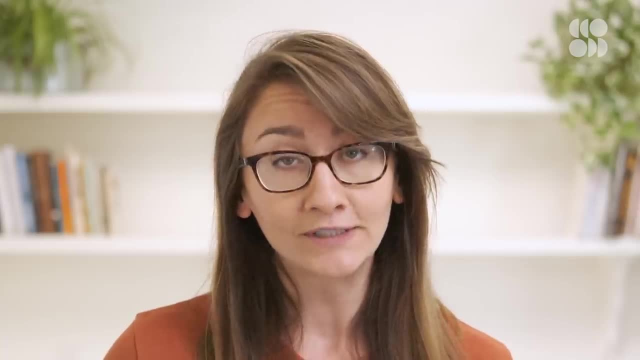 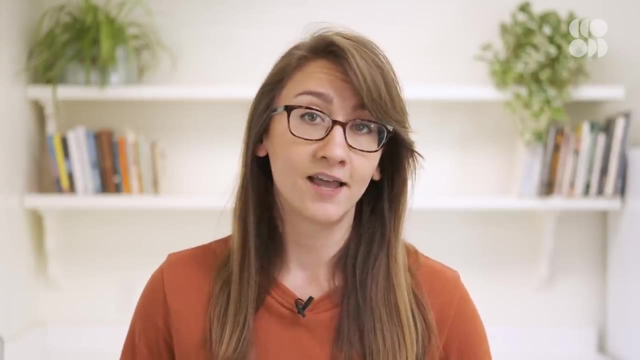 everything, which is exactly what physicists from around the world have been after. Which brings us back to the Brookhaven experiment In 2001,. the team published some surprising findings. Their measurement of the muon's g-factor deviated from the standard model's prediction. 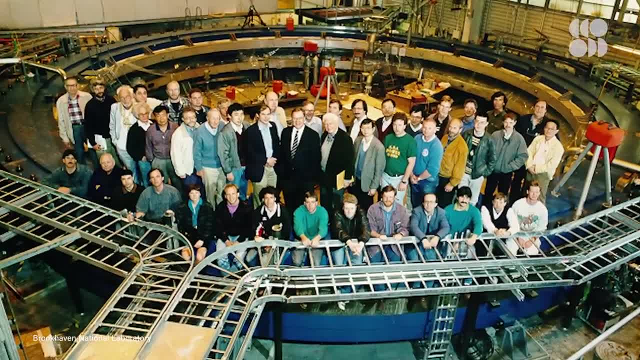 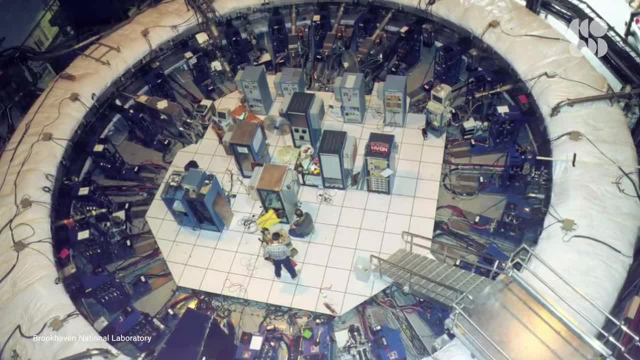 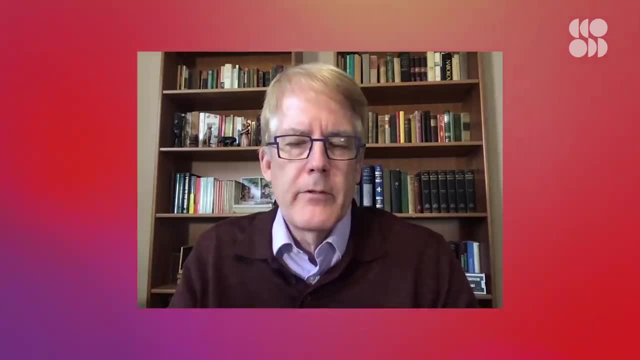 and nothing could account for the difference. Instead of finding a g-factor slightly above two, as the standard model had predicted, they found a g-factor that was off by nearly three standard deviations. The Brookhaven experiment was a big surprise. It made a lot of people think that maybe there's something we really don't understand either. 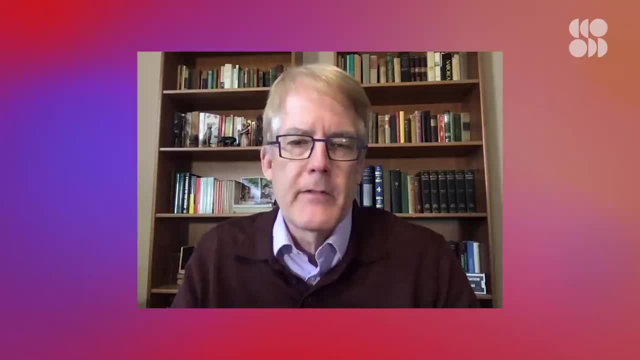 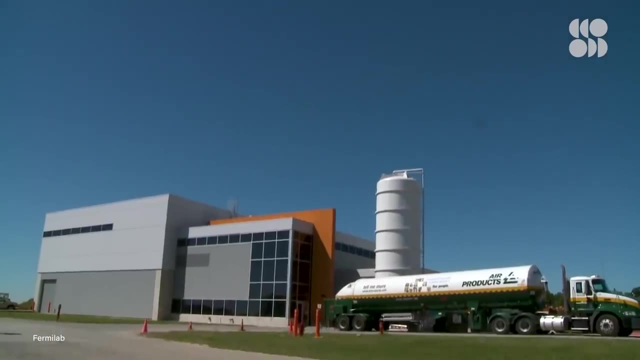 about particle physics or about how to do these kinds of experiments. So the physics community decided that the only way to confirm these findings was to take that measurement. again. Led by Fermilab, the muon g-2 experiment cast its first beam of particles back in 2017,. 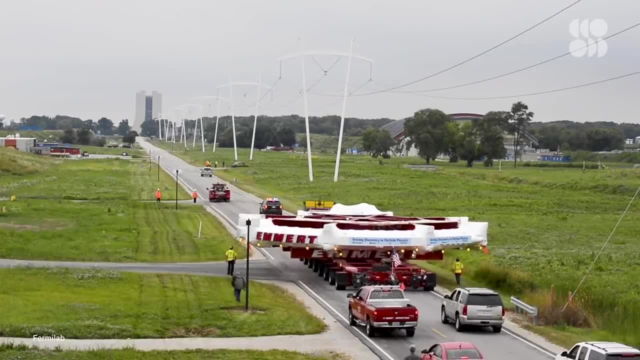 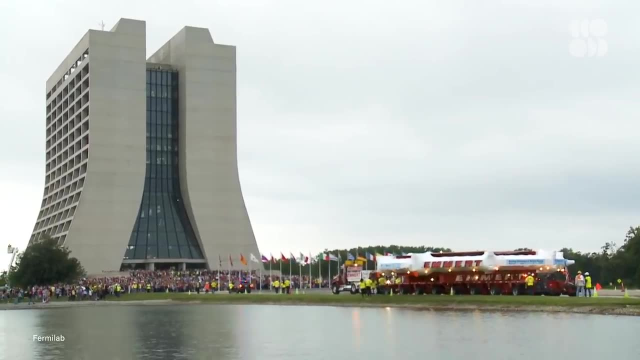 and has been searching for the muon's g-factor ever since. We decided to combine the experimental technique by moving the magnetic ring from Brookhaven National Lab all the way to Fermilab. Fermilab's accelerators were also used to measure the muon's g-factor. 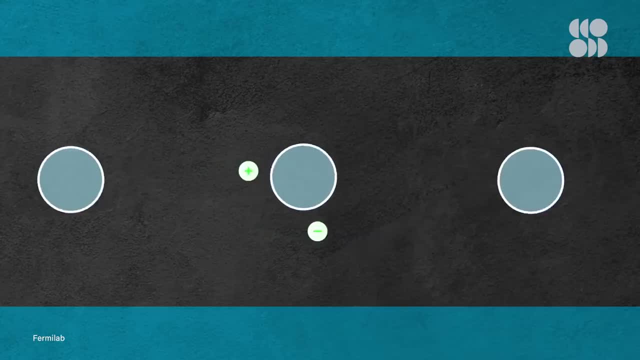 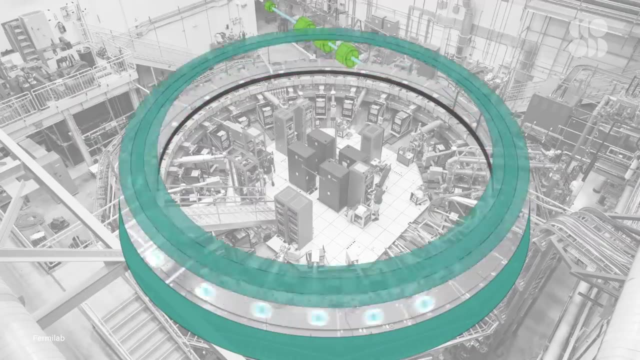 The accelerators first blast particles into a giant ring where they decay into muons. These muons then travel to a second ring where they spin and start to wobble in reaction to the ring's powerful magnets. By comparing measurements of this wobble with the ring's magnetic field, the team is able 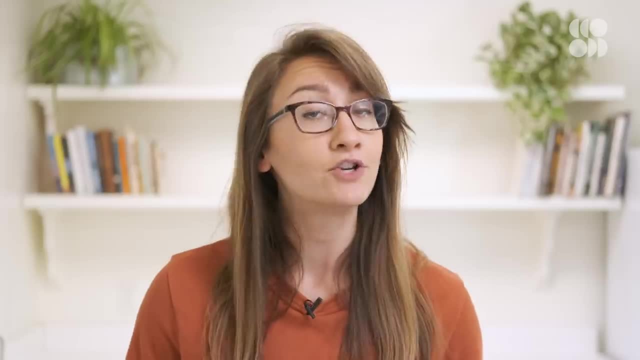 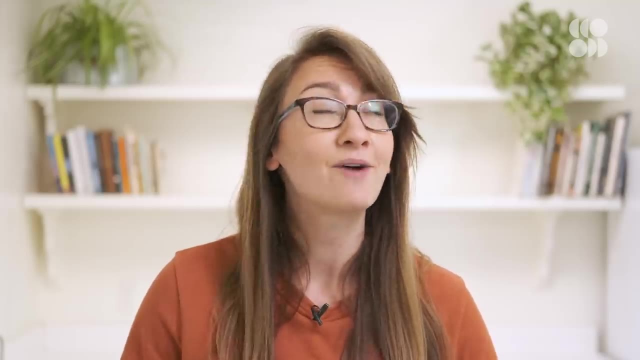 to walk away with a measurement of the magnetic moment with a precision of 0.14 parts per million. At this level of precision we get a window into the world of muons that we've never had before And a more specific number to compare our theoretical predictions with.